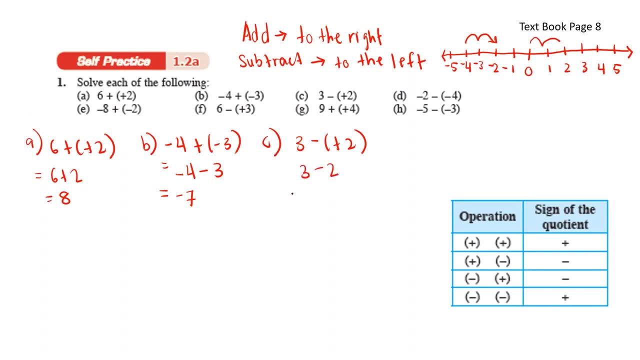 and negative. you get negative: 3 minus 2.. 1. Negative, 2 minus negative. 4. Negative and negative: you get positive. So negative: 2 plus 4, you get negative, 2 plus 4.. 1,, 2,, 3,, 4. You get 2.. 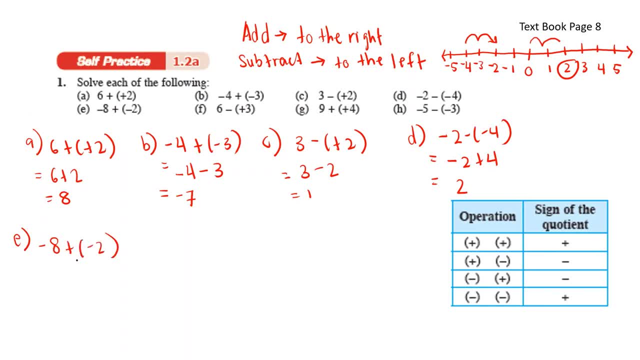 Negative 8 plus negative 2.. Positive and negative: you get negative. So negative 8 minus 2 will move to the right, So you get 2.. We get 2.. two steps to the left from negative 8, you'll get negative 9, negative 10.. 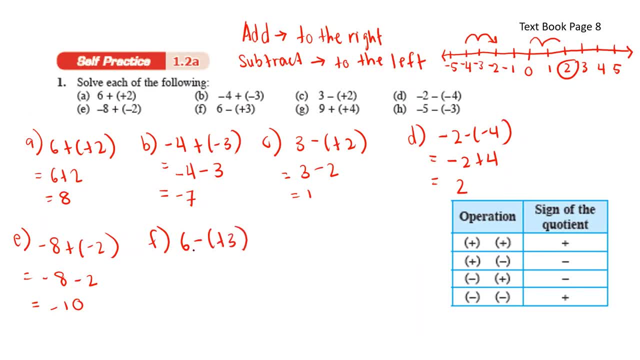 6 minus positive, 3. Positive and negative: you get negative. So 6 minus 3, you get 3.. 9 plus positive, 4, you get positive. and positive is positive. So 9 plus 4, you get 13.. Negative, 5 minus negative, 3. Negative and negative: you get positive. So 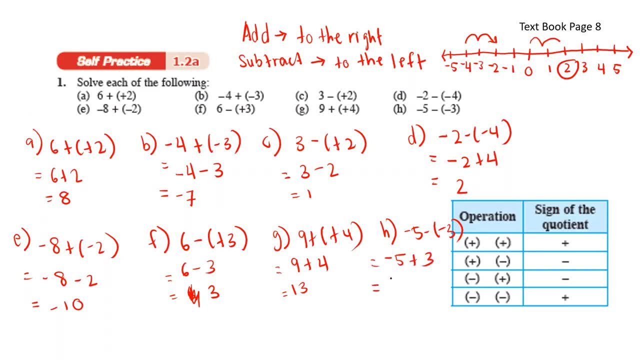 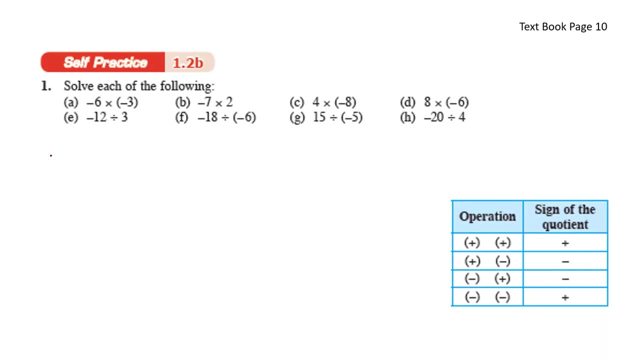 negative: 5 plus 3,, you get negative 2.. Take a look at self-practice: 1.4.. Negative 6 times negative, 3. So negative and negative will result in positive. So we get positive 6 times 3, 18.. Negative: 18.. 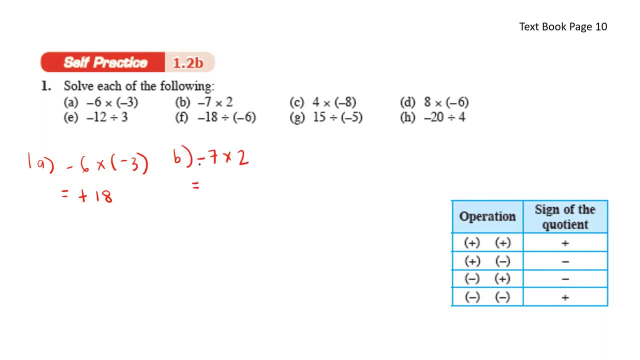 Negative 7 times 2.. Negative and positive: you get negative 7 times 2,, you get 14.. Negative 4 times negative: 8. Positive and negative: you get negative. So negative 4 times 8, you get 32.. 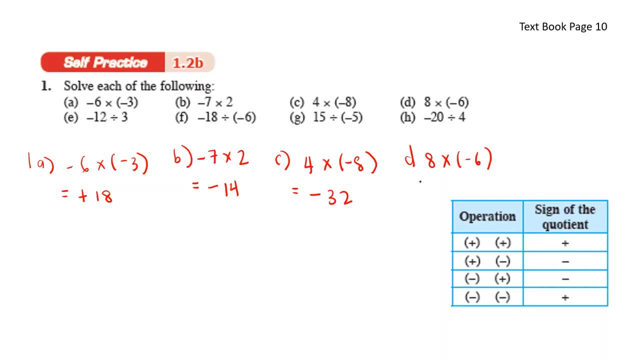 8 times negative. 6.. Positive and negative: you get negative. So negative 8 times 6, 48.. Negative: 12 times negative. Right, 12 divided by 3.. Negative, positive: you get negative. 12 divided by 3, you get 4.. 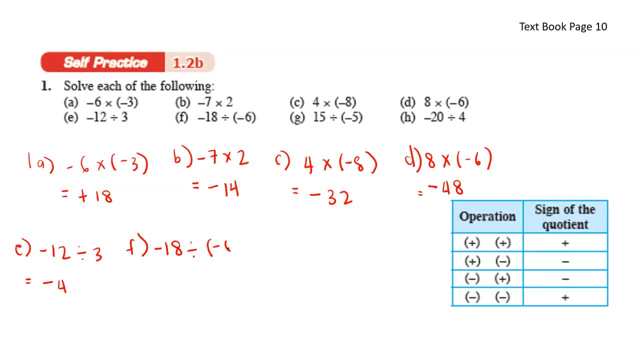 Negative: 18 divided by negative, 6. Negative and negative: you get positive. 18 divided by 6, you get 3.. 15 divided by negative: 5. Positive and negative: you get negative. 15 divided by 5, you get 3.. 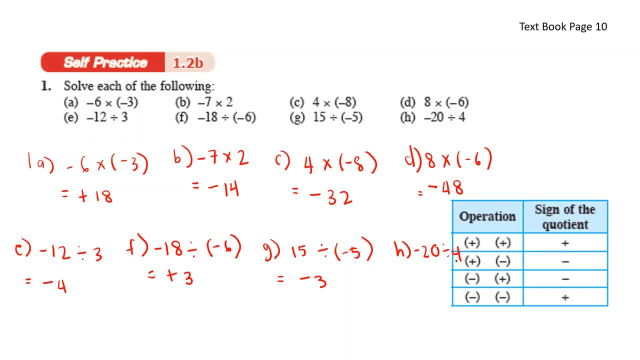 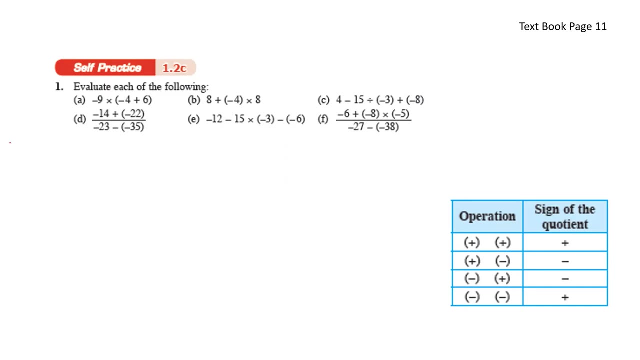 And lastly, negative 20 divided by 4.. Negative and positive: you get. negative. 20 divided by 4, you get 5.. Next let's take a look at self-practice: 1.5.. 2.2c. Evaluate each of the following. 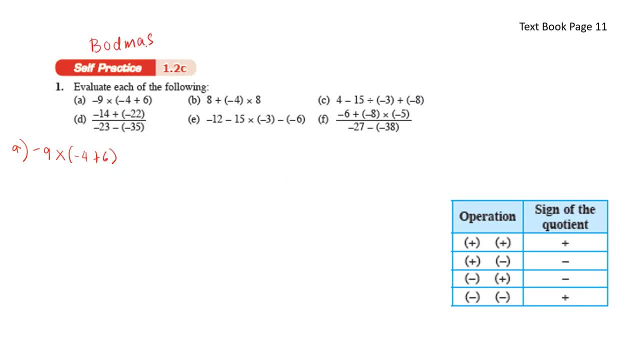 According to the BODMAS rule, operations within the bracket comes first. So let's start with the operations within this bracket. Negative: 4 plus 6, you get 2.. So negative 9 times 2.. Negative and positive: you get negative. So 9 times 2, you get 18.. 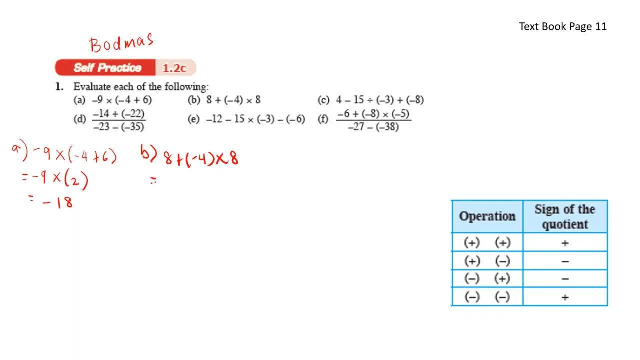 8 plus negative 4 times 8.. Here there are two operations, which is addition and multiplication, And according to the BODMAS rule, multiplication comes first. So following that, let's do negative 4 times 8.. 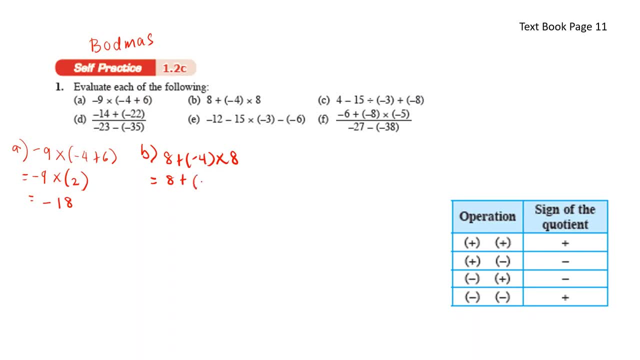 So positive and negative. you get negative. 4 times 8, you get 32.. So you get negative 32.. 8 plus negative 32 will result in 8 minus negative 32, because positive and negative is negative. 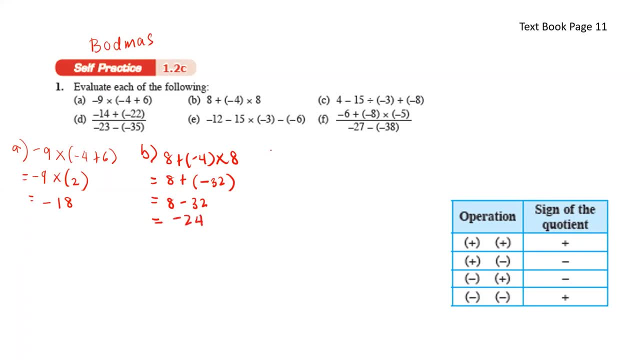 And you'll get negative 24.. Form minus 15, divide by negative 3 plus negative 8.. First we will start with division, So it will be 4.. Negative 15, divide by negative 3, you get negative and negative, you get positive. 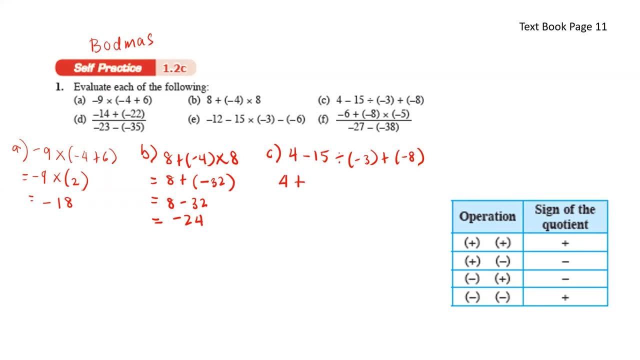 15 times 15, divide by 3, you get 5. Plus negative 8.. So 4 plus 5, you get 9.. Positive and negative: you get minus 8, resulting in 1.. For fraction operations, always do numerator and denominator separately. 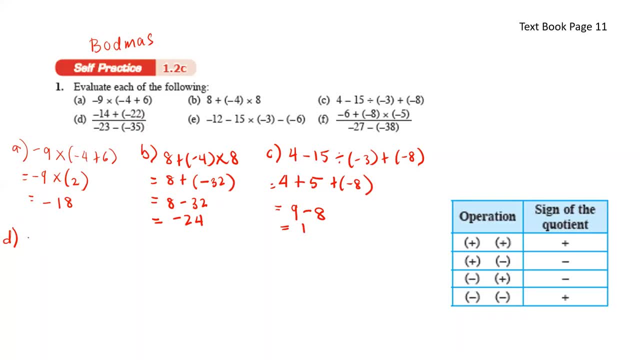 Then in the end solve the fraction. So here we'll start with negative 14 plus negative 22,. the numerator over negative 23 minus negative 35. So here we get positive And negative, which is negative. 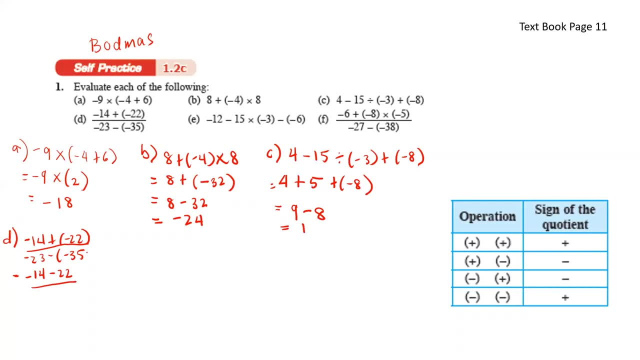 So negative 14 minus 22,. over negative negative you get positive. So negative 23 plus 35. So here we get negative 36 over 12,, resulting in negative 3.. Next negative 12,, negative 15.. 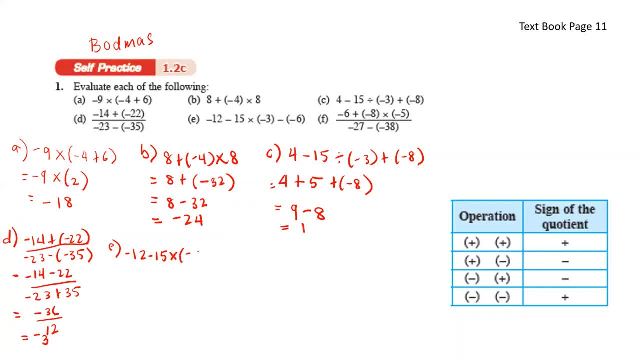 Minus negative, minus 15,- sorry times- negative: 3, minus negative: 6.. So here we will do multiplication first, So we'll get negative 12.. Negative negative: you get positive. 15 times 3, you get 45.. 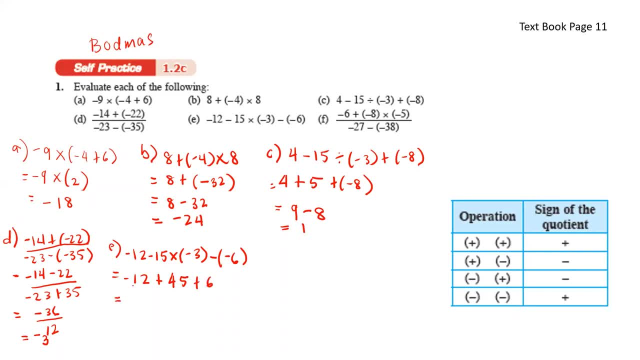 Negative, negative, you get positive. So negative: 12 plus 45, you get 33. Plus 6. You get 39.. And lastly, as I said earlier, for fractional operations you start with numerator and denominator separately. 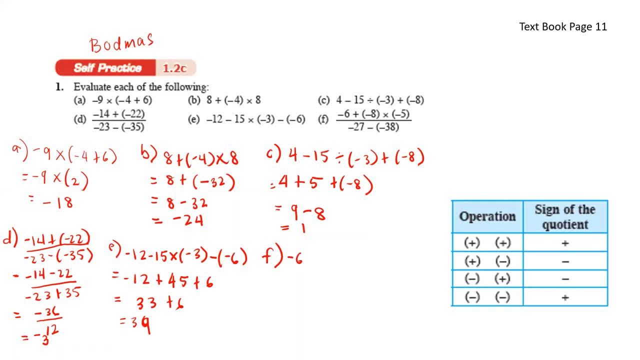 Then solve the fraction. So negative 6 plus negative, 8 times negative 5 over negative, 27 minus negative 38.. So here we get negative 6.. Negative, negative: we get positive. So positive plus positive 40 over negative negative, you get positive. 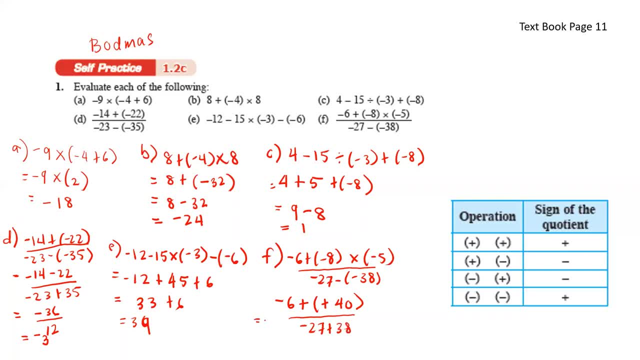 So negative: 27 plus 38.. So here we get. this will result in a positive. So negative 6 plus 40 will give you 34 over 11.. So here you get: 3, 1 over 11.. 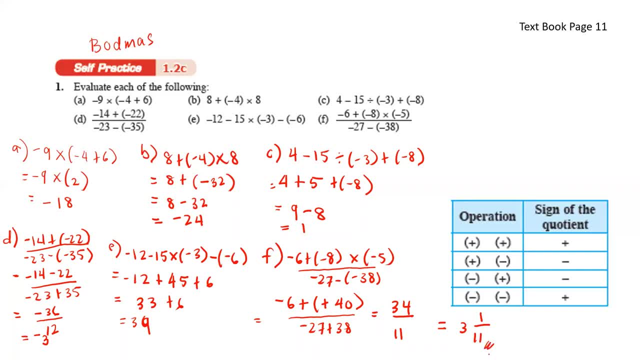 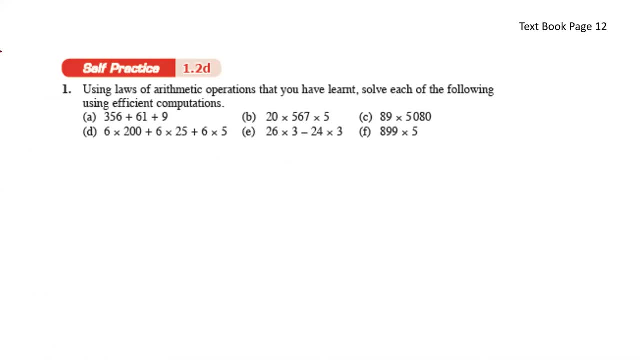 Moving on to self-practice. 1.2d, Using laws of arithmetic operations that you have learned, solve each of the following using efficient computations: 356 plus 61 plus 9.. So first, 356 plus 61,, you get 417. plus 9,, you get 426.. 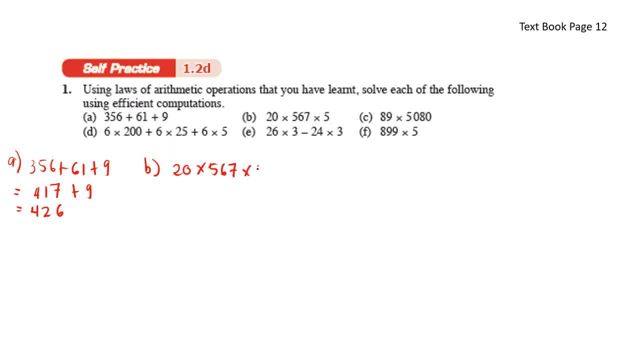 20 times 567 times 5,, you get 11,340 times 5.. You get 5, 56,700.. 89 times 5,080,, you get 452,120.. Okay, 6 times 200 plus 6 times 25 plus 6 times 5.. 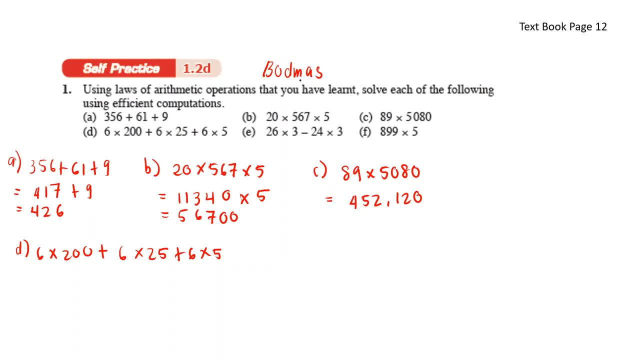 So once again, according to the BODMAS rule, multiplication comes in the form of the following: Multiplication comes before addition. So here we'll do all the multiplication operations first. So we'll do 6 times 200, you get 1,200 plus 6 times 25,, 150 plus 30.. 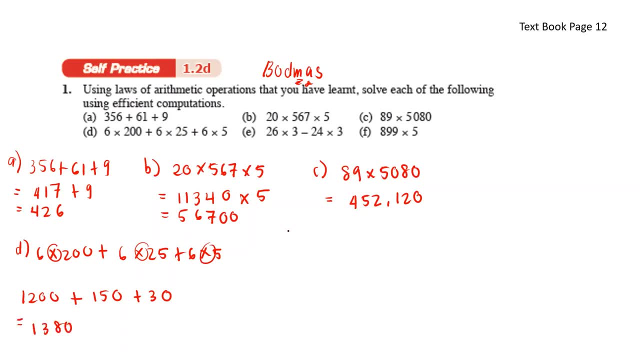 You get 1,380.. Next 26 times 3.. Minus 24 times 3.. In the BODMAS rule once again multiplication comes before subtraction, So we'll do the multiplication operations first. So here we have 26 times 3, 78.. 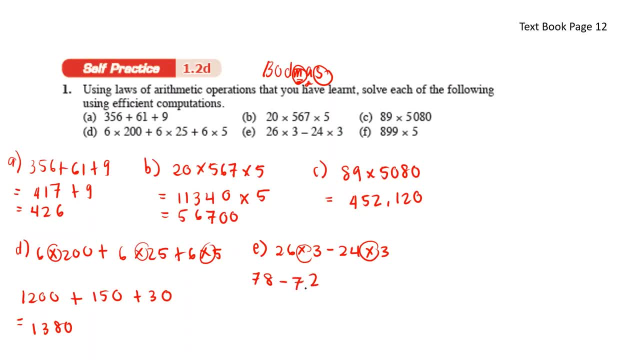 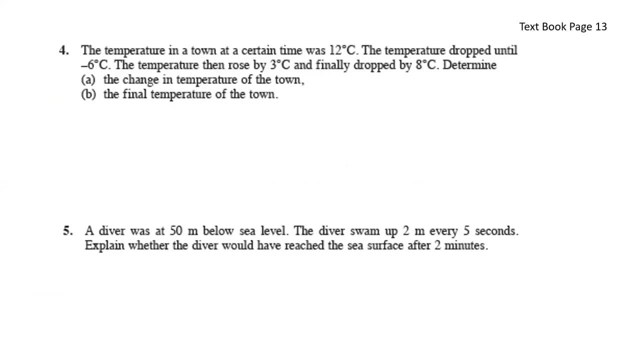 Minus 24 times 3,, 72,, you get 6.. And lastly, 899 times 5,, you get 4,000.. 4,495.. Okay, guys, Next let's do Mastery Q 1.2, number 4.. 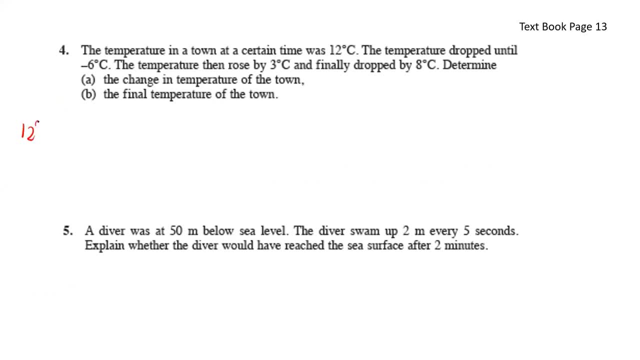 The temperature in a town at a certain time was 12 degrees Celsius. The temperature dropped until negative 6 degrees Celsius. The temperature then rose by 3 degrees Celsius And finally it dropped by 8 degrees Celsius. Okay, Determine the change in temperature. 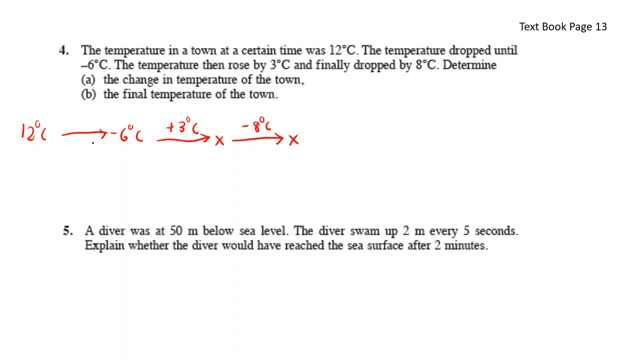 The temperature of the town. So from 12 degrees Celsius to negative 6, we have a difference of negative and negative. you get positive. So 12 plus 6, you get 18 degrees Celsius. However, since it mentioned here as a drop in temperature, it will denote a negative. 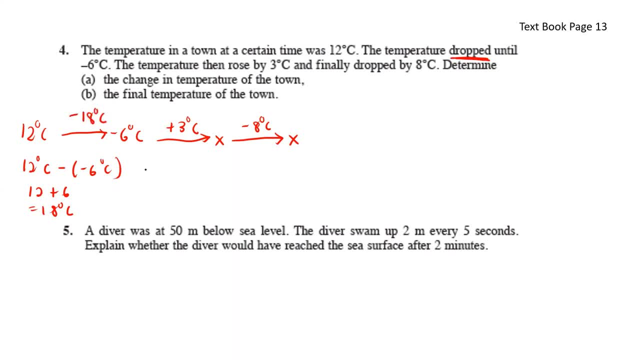 18 degrees Celsius. Okay, negative. So in order to calculate the change in the temperature, we'll have to add a negative 18 plus 3 plus negative 8 gives us negative. 18 plus 3 gives us negative. 15, positive. 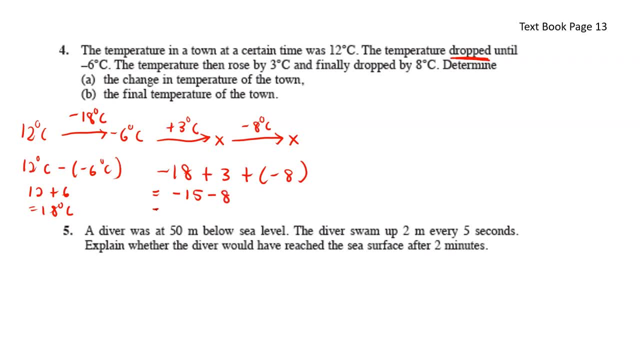 and negative gives us negative 8.. So negative 15 minus 8 gives us negative 23 degrees Celsius And B the final temperature of the town. So the final temperature would be this temperature. Now let's look: Negative 6 degrees Celsius plus 3 degrees Celsius gives us this one as negative 3 degrees. 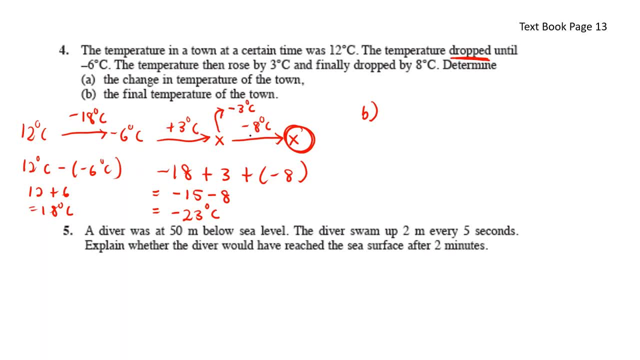 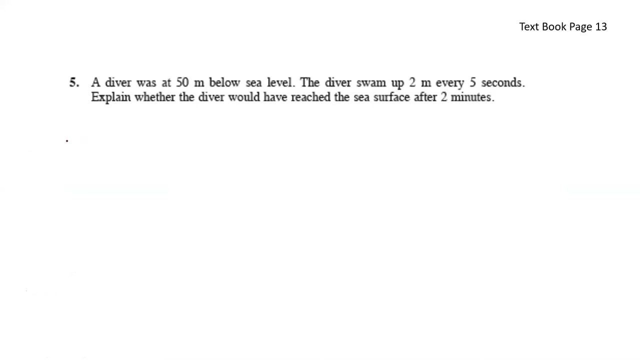 Celsius. So once it drops means negative 3 degrees Celsius. minus, sorry, minus 8 degrees Celsius gives us negative 11 degrees Celsius. So this will be the final temperature of the town. A diver was at negative 50, was at 50 meters below sea level. 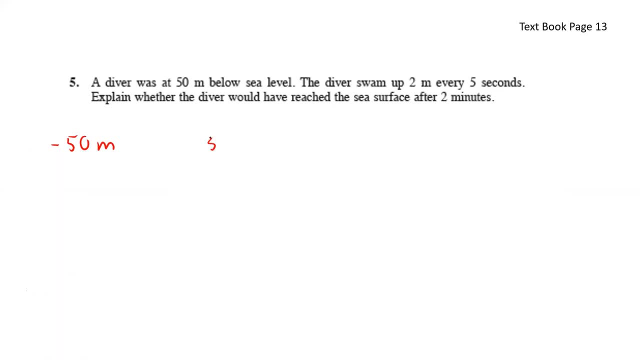 The diver swam up by 2 meters every 5 seconds. So for every 5 seconds we have 2 meters. Explain whether the diver would have reached the sea surface after 2 minutes. Okay, So with 1 minute we have 60 seconds. 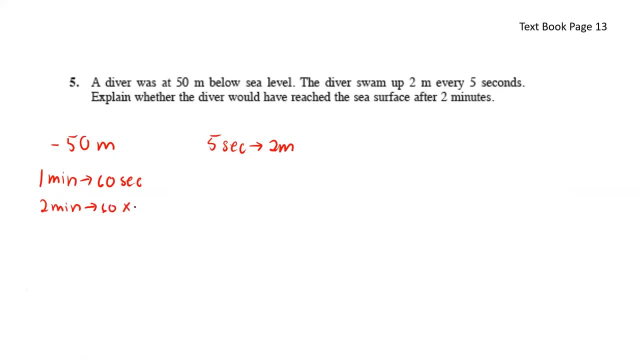 For 2 minutes that would be 60 times 2, 120 seconds. So if every 5 seconds he moves up by 2 meters for 120 seconds, let's calculate the distance he swam up. So that would be 120 over 5 times 2 meters. 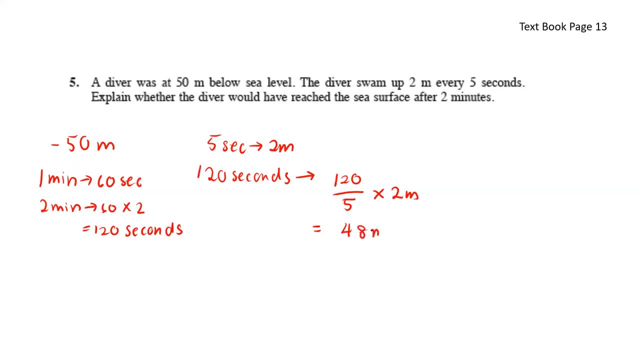 So that would give us 48 meters. Let's see whether he managed to reach the sea surface. So negative 50 meters, which is his current position, plus 48 meters that he swam upwards for 120 seconds, gives us negative 2 meters, which means he did not reach the surface. 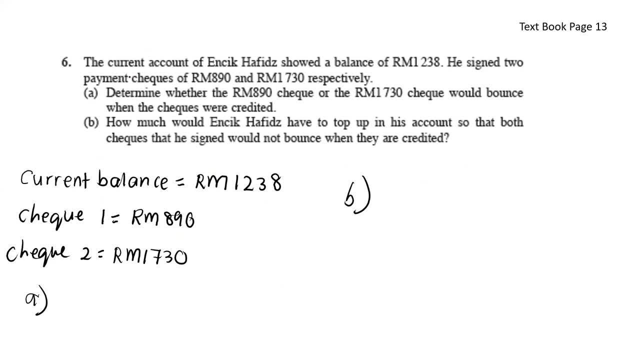 The current account of Encik Hafiz shows showed a balance of our current position. This is the balance for RM1238.. He signed 2 payment cheques of RM890 and RM1730, respectively. Determine whether the RM890 cheque or the RM1730 cheque would bounce when the cheques were credited. 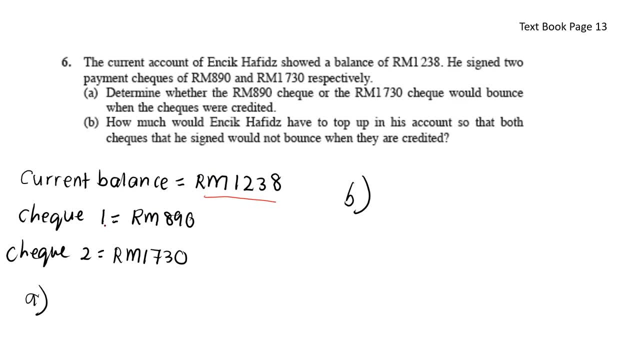 Okay. So, if this is the current balance, if Encik Hafiz would like to make a cheque payment, RM890 is sufficient, because it is still within this amount. However, the second cheque, which is RM1730, will bounce as it is more than the current balance amount. 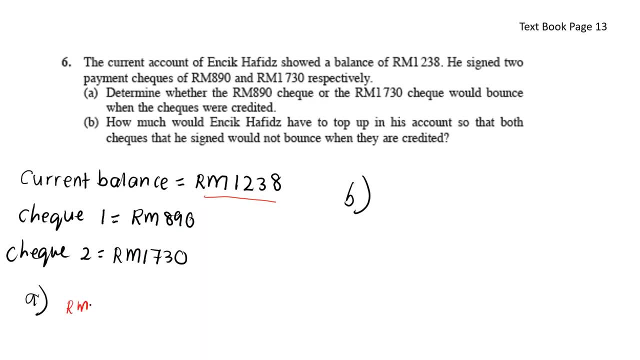 So the answer for A would be the RM1730 cheque. For B, how much would Ajit Hafez have to top up in his account so that both cheques that he signed would not bounce when they are credited? Okay, so currently we have RM1238.